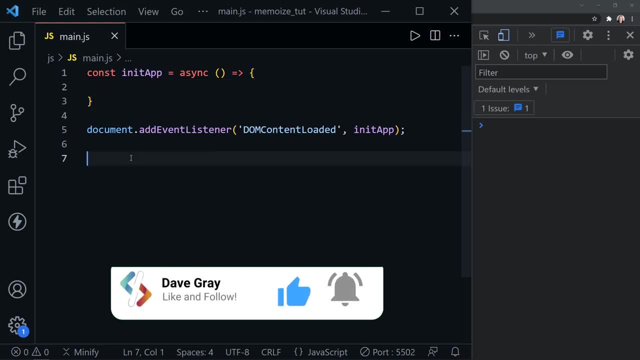 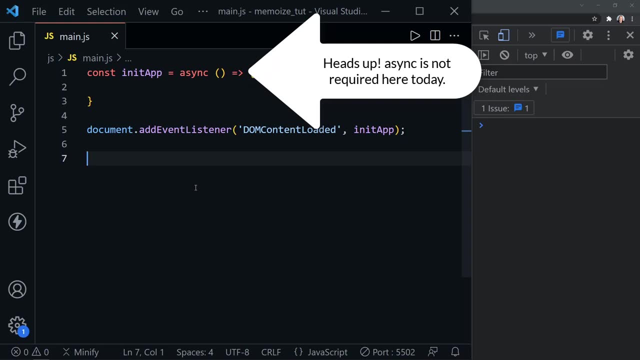 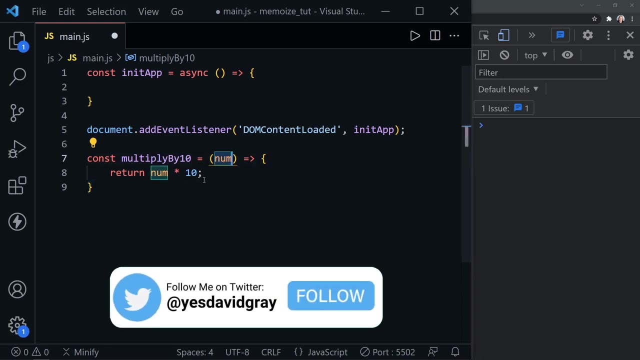 here. It doesn't have anything in it yet, but that's kind of what we would do with a vanilla JavaScript web app. So to demonstrate memoization, I'm first just going to paste in a very simple function. We see multiply by 10. here It's passed a number. Whatever number is received as a 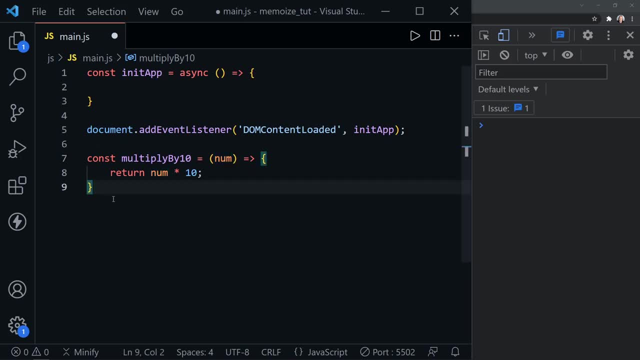 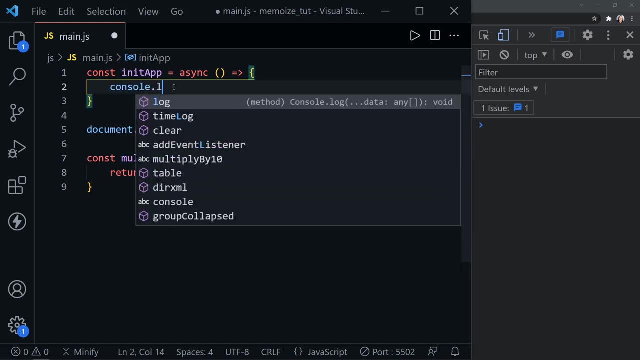 parameter is multiplied by 10, and the result is returned. So what I want to demonstrate with this- and I'll need to log to the console the results- We'll say consolelog, We'll call the function and I'm going to go ahead and pass in the number 10 as well. and now I'm going to copy this line: 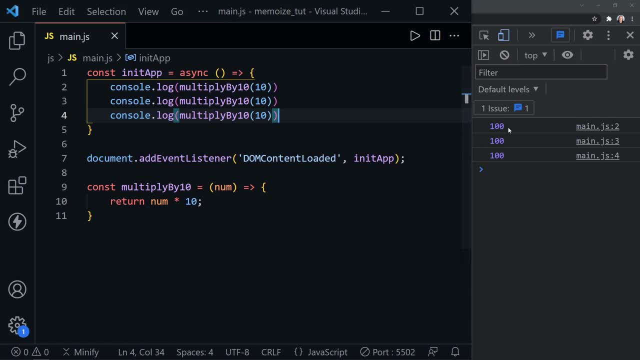 down a couple of times and save, and we see 100 three times in the console. What I'm demonstrating is, even though it calculated the result the first time, it had to recalculate the second time and it had to recalculate the third time. Now this is a very simple function, but imagine if 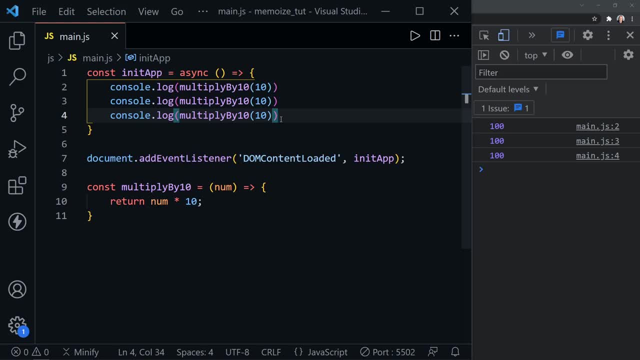 this was a process-intensive function and it took a while to calculate. This would be very inefficient. It's already calculated the result. Well, that's where memoization comes in. So now let's create a memoized multiply by 10, and I'll do that right underneath here. So we'll say: 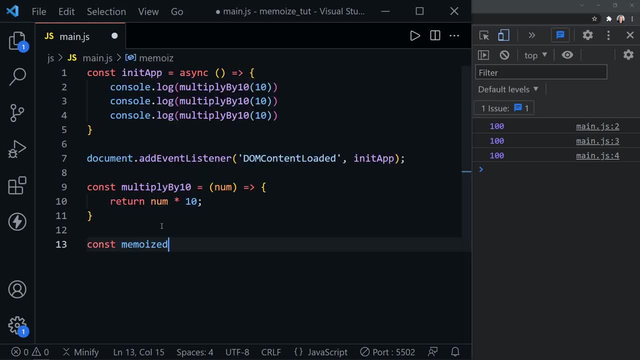 const memoized, multiply by 10,. and now inside, the first thing we're going to do is create a closure, and that's what will restore our cache. That's where we want to keep the results after we've calculated them. After that, and if you're familiar with closure already, you'll know. 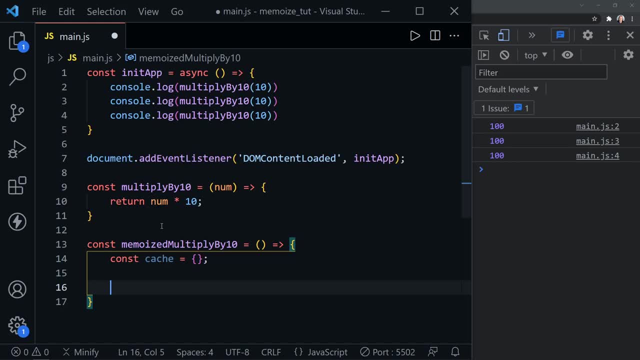 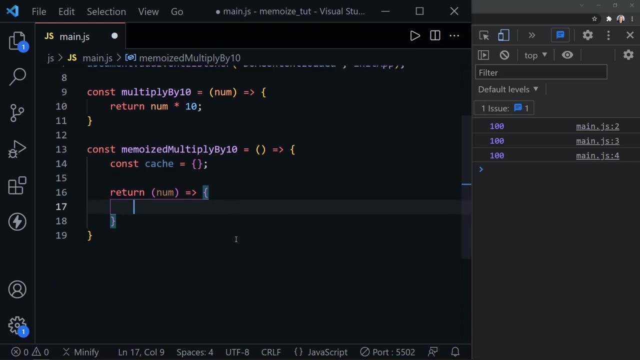 what I'm going to do. If not, you'll want to watch my tutorial on closures, but here I'm going to return an anonymous function and this is what receives the number parameter. and now, inside of this anonymous function, I'll scroll up to give us a little more room. we're going to check our 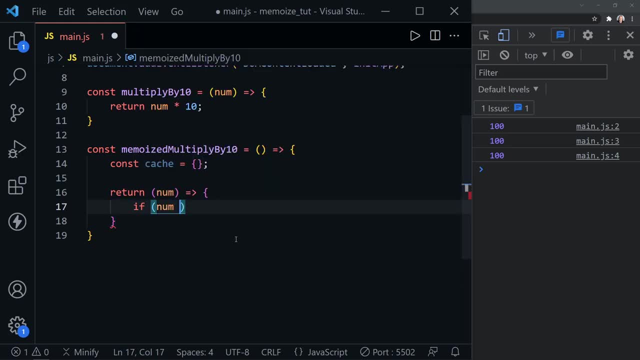 cache. So we'll say: if the num that's received as a parameter is in the cache, then we're just going to retrieve that result from our cache. So I'm going to log the cache to the console here, just so we know that's. 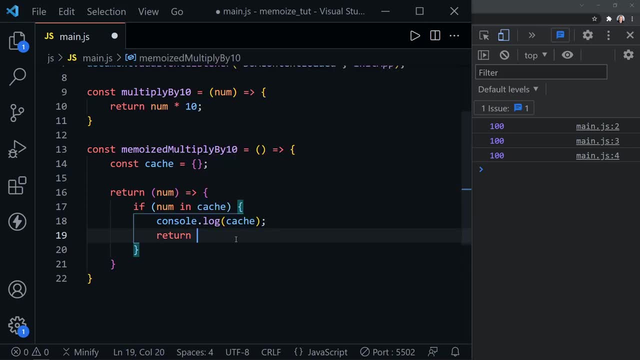 what we're doing as we walk through this, and then we return the cache and, of course, we refer to the key, which will be the number received, as the parameter, and, of course, keys are stored as strings, but we can refer to it this way. Now we don't really need a 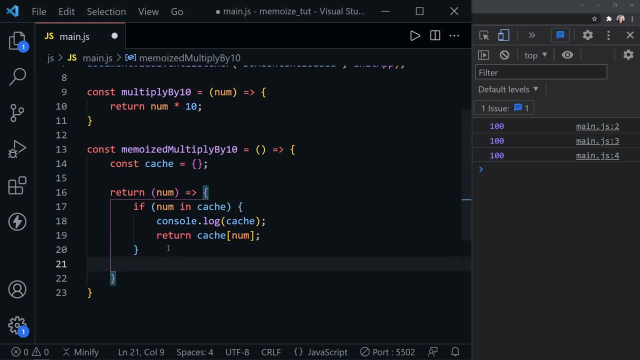 return else here, because that's a return. so if the number's in the cache it's going to return there and the function will be done. If not, it will just come down here anyway and we'll define the result and here we'll go ahead and calculate If this has never been called with the parameter. 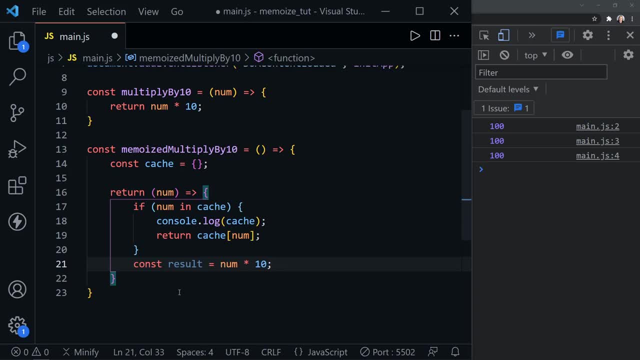 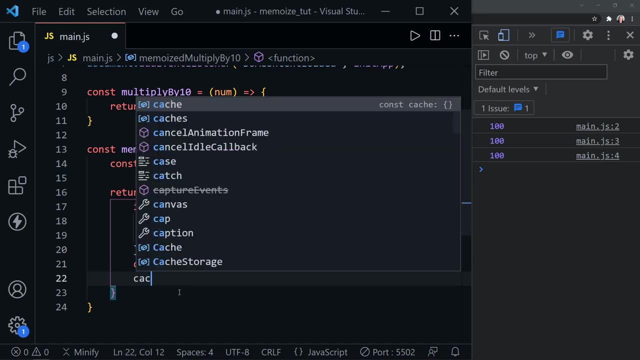 passed in, it will need to calculate it before it can store the result in the cache, which is essentially memoizing the answer, so it can refer to it quickly next time, and then that's exactly what we'll do after we calculate the result. 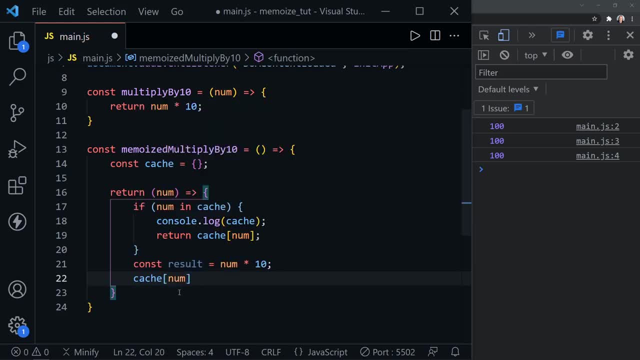 We'll store that result, so cache with the num, as the key here is going to be equal to the result. and then, of course, we need to return the result, and that pretty much sums it up Now, when we call this, 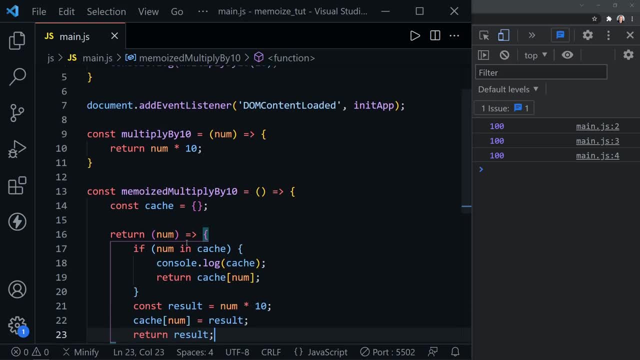 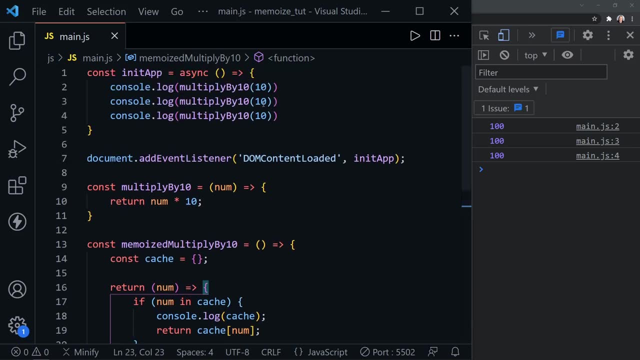 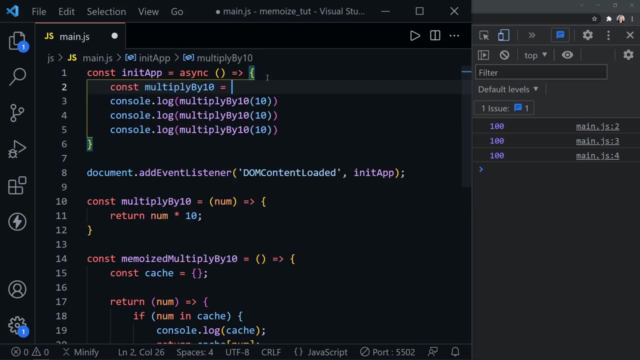 into action. it will be just a little different than you might expect. so instead of calling multiply by 10 and passing in the number right away, what we need to do up above is say: const multiply by 10 is equal to our memoized multiply by 10 and call that. and that's because. 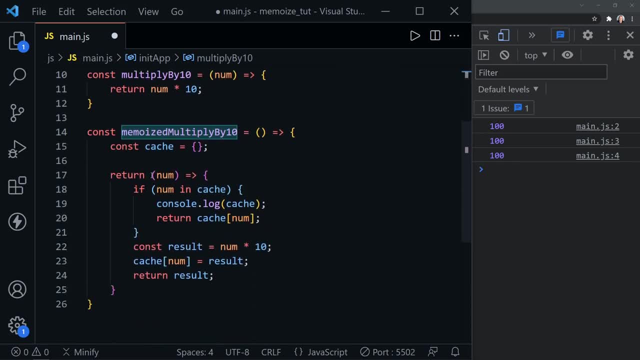 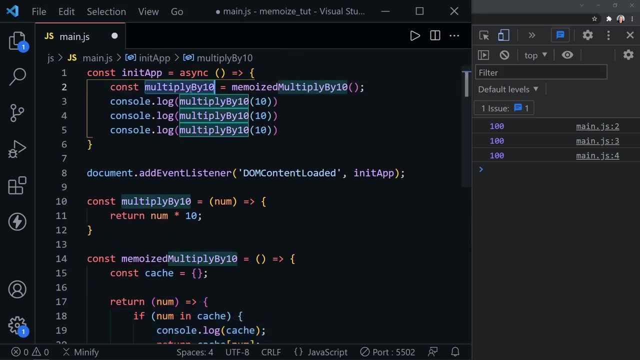 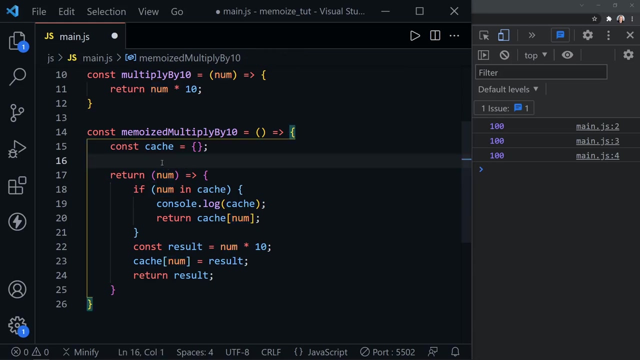 our memoized multiply by 10 will return this anonymous function, and then we're able to call this function with our multiply by 10 and pass in the parameter whichever number we want, which we have right here. but the bonus is, with the closure, this anonymous function is going to be. 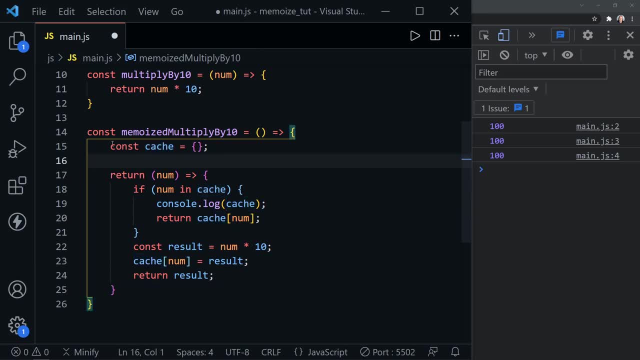 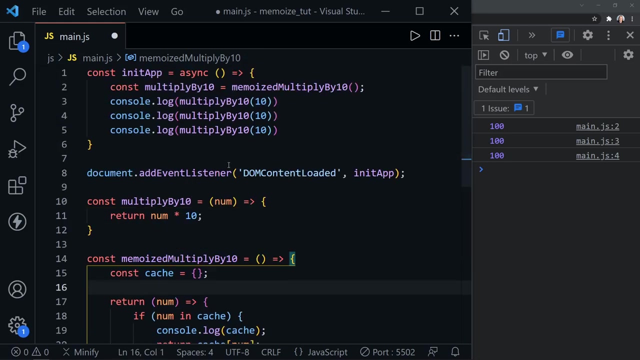 referred to what's ever stored in this private cache. It's only available because of the scope here of this function through a closure. Once again, if you're not familiar with closures, check the link in the description below. but we can refer to the cache and we can call it. 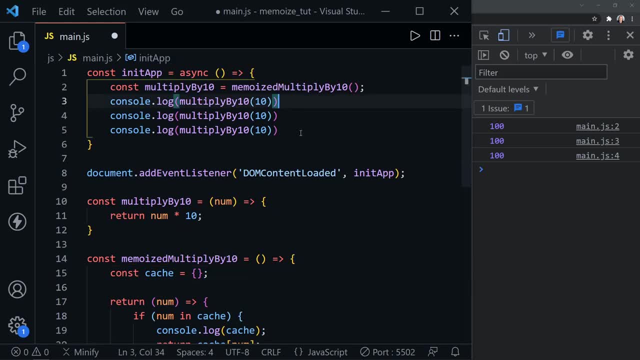 with multiply by 10, so we're going to do that three times and let's look at the result now. when I save, We get the calculated result first and then the second time. we are logging the cache to the console and you can see the key here is 10, which is the 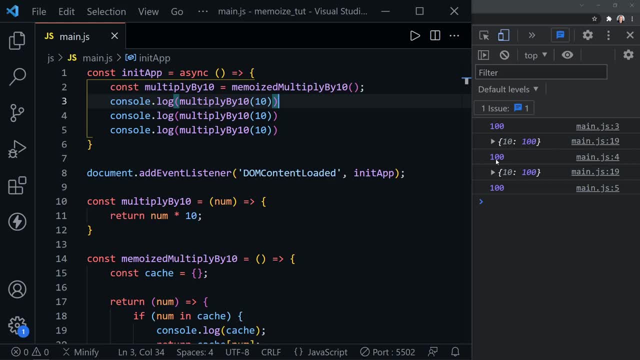 parameter we passed in and here's the result, and then, of course, it provides the result right away, and then we called it a third time and the same thing happens, because the result is stored in the cache. Now, if I copy this down again, but change the number, and I'll say I'll pass in the 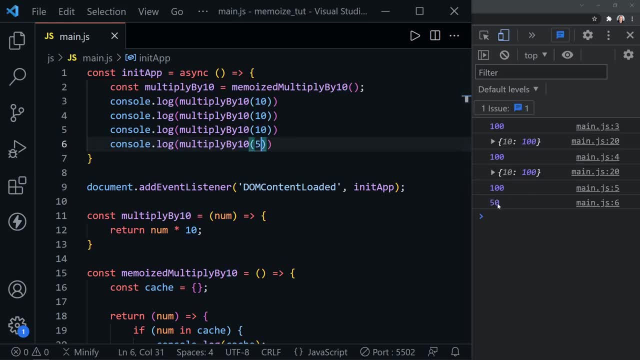 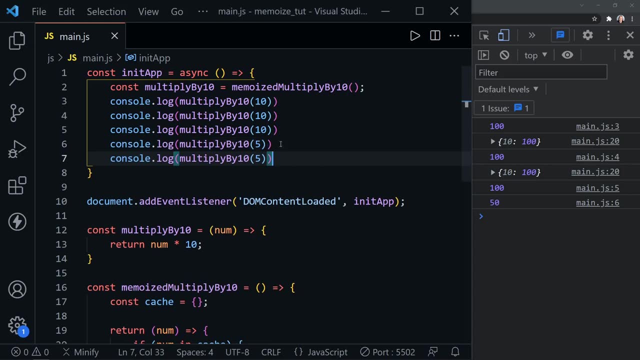 number five and save. you can see the cache is not logged because it had to calculate this result. It didn't already have that in the cache, but if we do it one more time and I save now you see our cache and it has the result for five and the result for 10, so it can refer to. 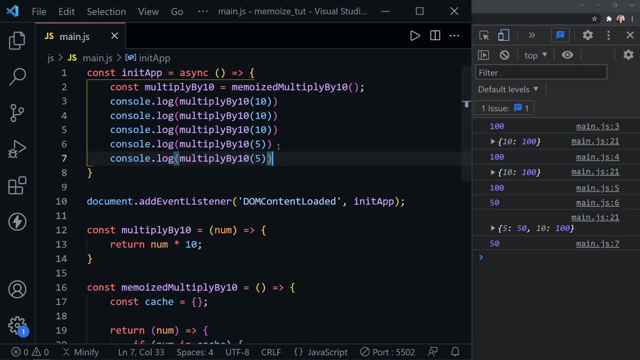 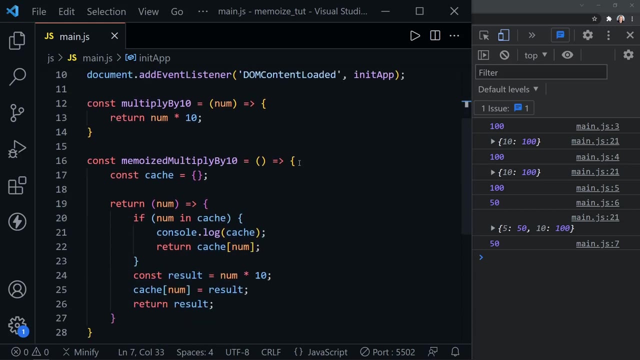 that and deliver it immediately. Now again, these are not intensive functions here, but imagine if the processing time did take a while. The second time around it would be instantaneous, and that's the benefit of memoization. Now let's look at how we can apply. 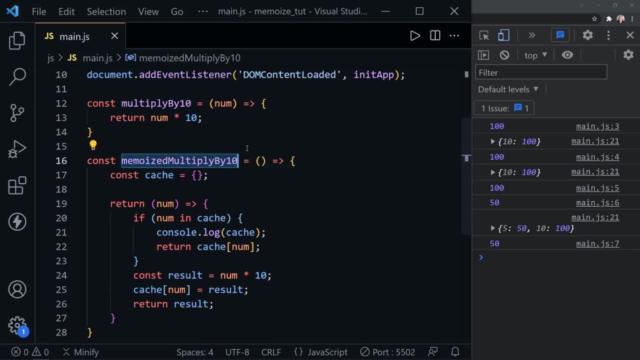 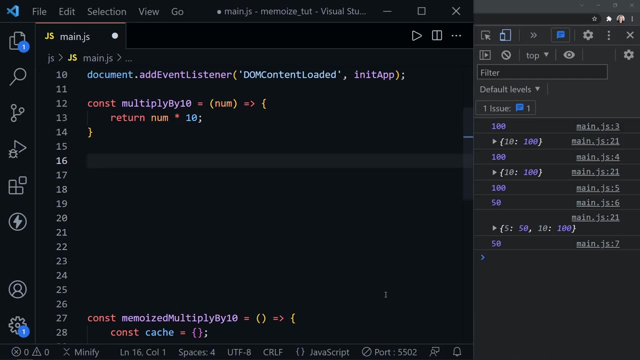 this without creating a separate function like this every time We can actually create a decorator function that will memoize any other function we pass into it. Okay, I'm going to make some room here and we'll create our new function that is a decorator that will memoize other. 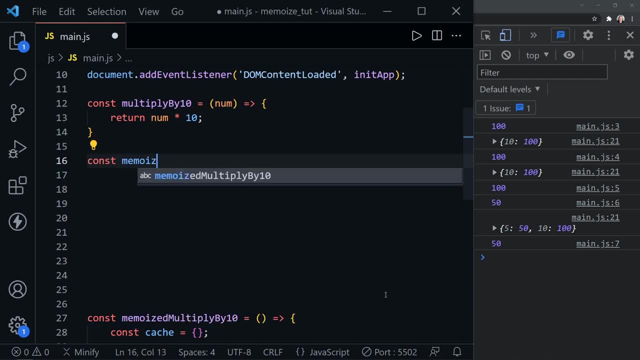 functions. so let's call this memoize, and then we'll accept a function as a parameter, because that's what decorator functions do. haven't watched my tutorial on decorator functions? I'll make sure to link to that below as well. Now what we do is create a cache, and this cache is set equal to an. 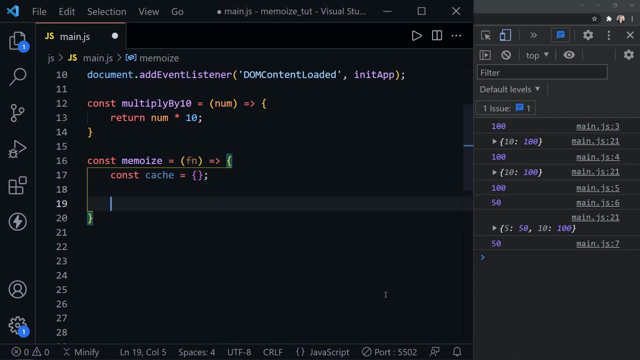 empty object. and now, if you are thinking about closure, that's exactly what I'm going to create here, because I am going to return a function and it receives the arguments. This is a rest parameter, by the way, and so these are just. however many parameters are passed in, or we refer to them as args, I could rename. 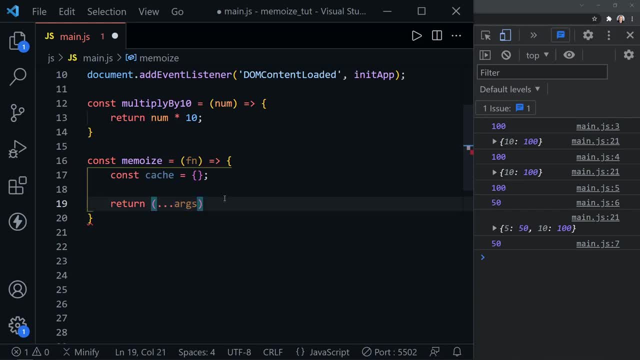 this params, if I wanted to, and it just ends up being an array of the parameters. So now we're returning this anonymous function and by doing that this creates a closure and the cache is available to this anonymous function through the lexical scope, and so we will access the cache and it's kind of a. 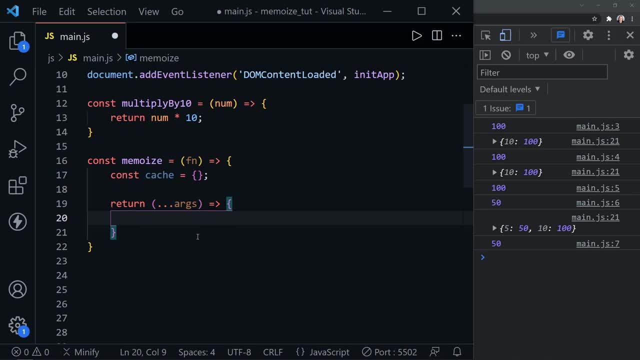 private variable here as well. because of that, That's how a closure works, and again, more of that is in my closures tutorial as well. So we're returning this anonymous function and the first thing we need to do is say if the args, which is this array of parameters that are passed in, or 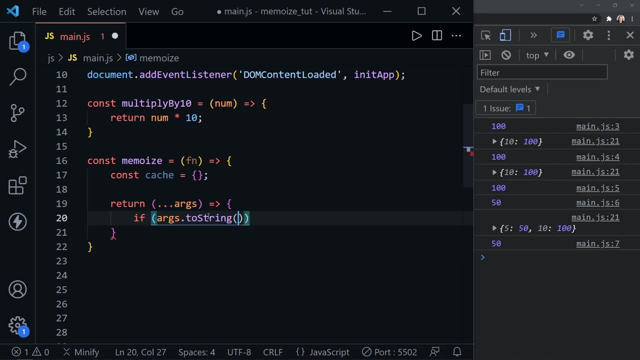 arguments, if you will, and we'll say toString, because we're going to refer to the key in the object and the key is typically stored as a string. If the key here defined by the args set to a string is in our storage cache, then we'll return our answer, just. 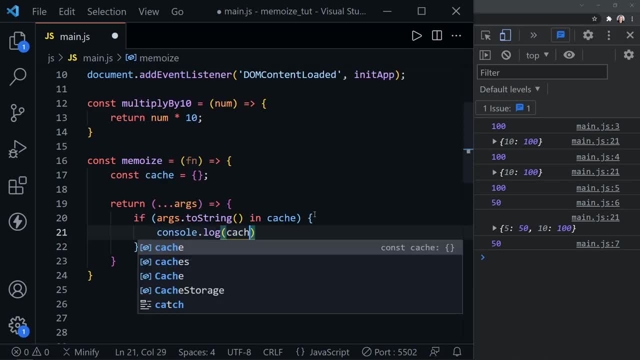 by referencing the cache. so i'm going to log the cache to the console so we know we're accessing the cache when this happens, and then i'm going to return the cache and then we'll reference the key in the cache object by args, dot to string. there we go, and now we don't need an else here, because 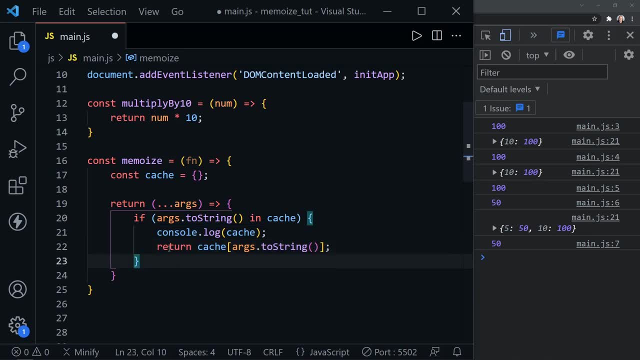 this is a return. so if this is true, we're going to return right here, but if it's not true, it'll skip all of this and it will just come down here and then we'll go ahead and call the function. so we'll set our result equal to the function and pass in the args which are the parameters. 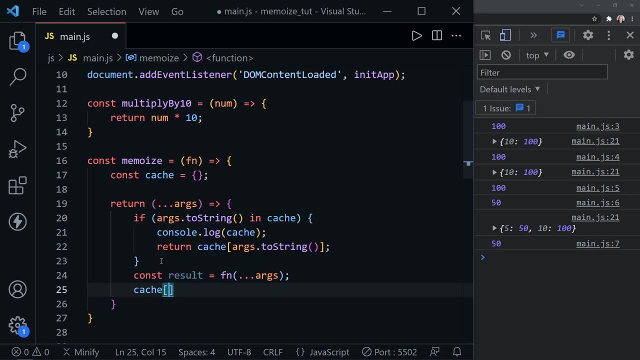 and then we'll take the cache and once again refer to that key by args dot to string, and then we'll set that equal to the result. so now, after we've calculated the function here, whatever it is supposed to do, whichever function we've passed in, after we've 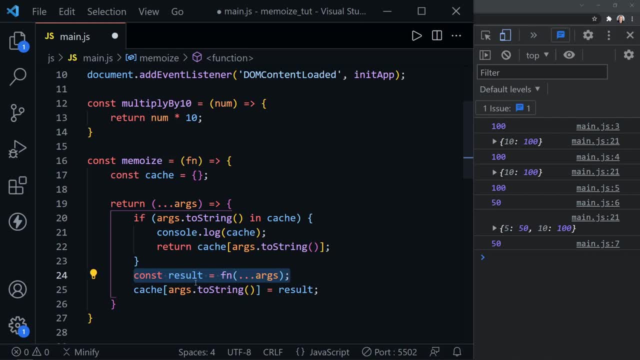 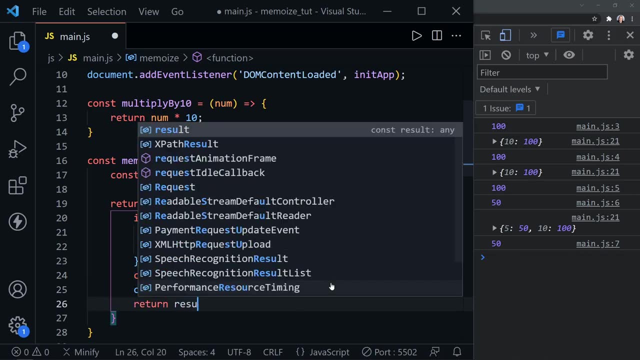 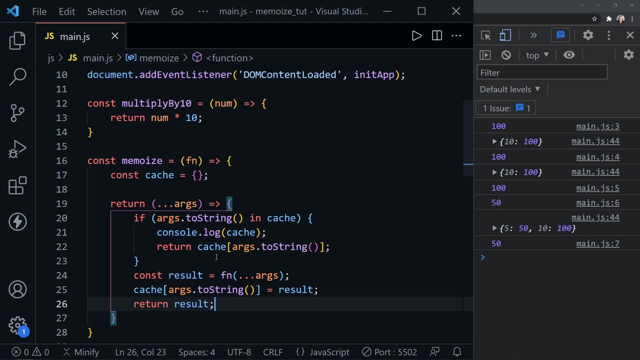 got the result. we store that in the cache, and that's why it won't take any time at all to look it up the next time, and then we'll just return the result here. so there's our complete memoized function that accepts another function and adds the memoized functionality to that. so now let's apply this to a couple of functions. 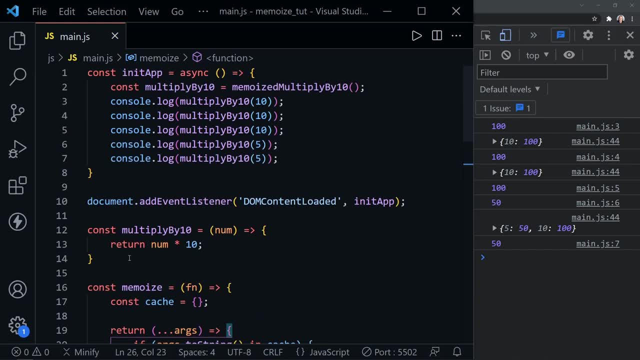 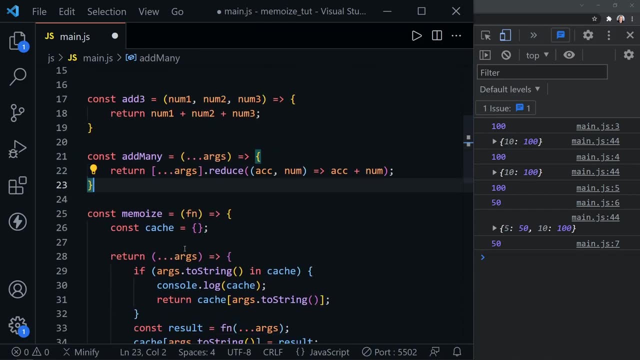 okay, i'll scroll back up now. we've already worked with multiply by 10, so let's do something different. it only accepts the one parameter as well, and our memoized decorator function will accept more than one parameter. that's why we have this array of arguments. so here you can see. 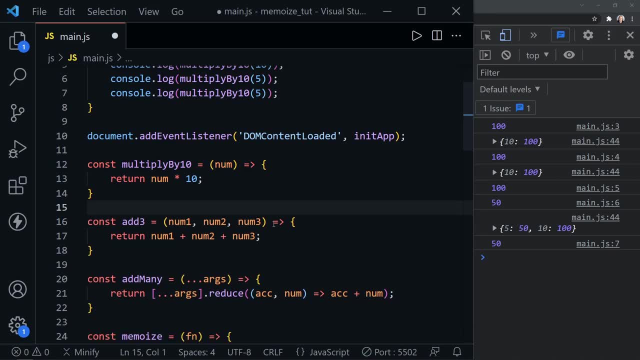 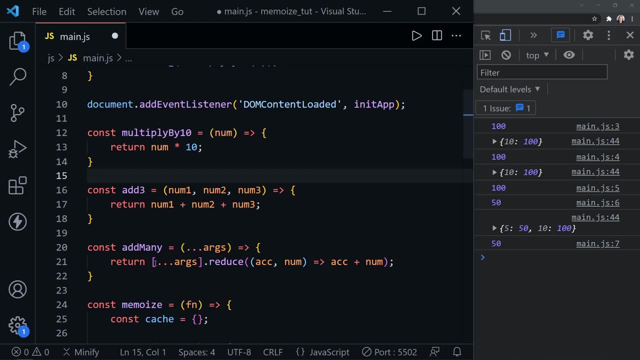 i've pasted in a function called add to the array of arguments and then we'll just return the result here: add three, and it has three parameters. and then i've pasted in a function called add many, and actually i'm putting the args in an array here, but i could just say args because it is already. 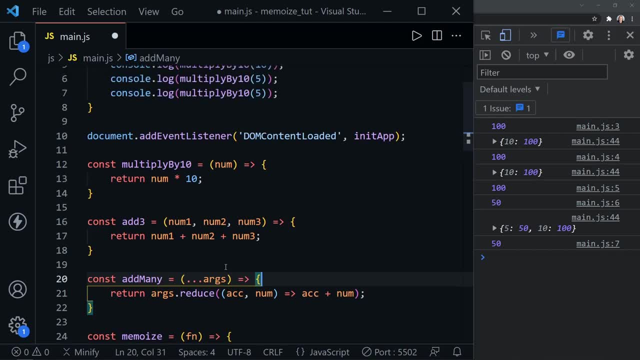 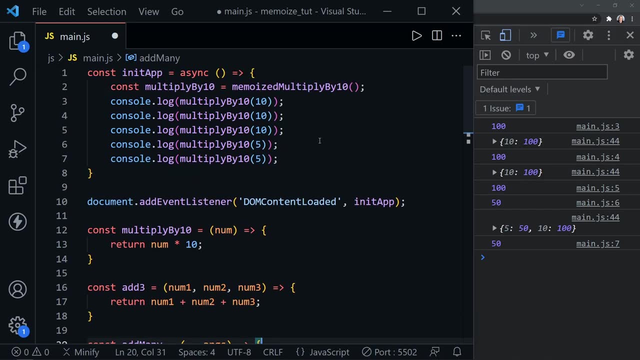 an array. so quick correction there, and now, up here, let's go ahead and apply our memoized to these functions. so first we'll just change this out and we'll get the same result. but we'll say: let's see memoized malt by 10, let's call it that, and then let's call over here. 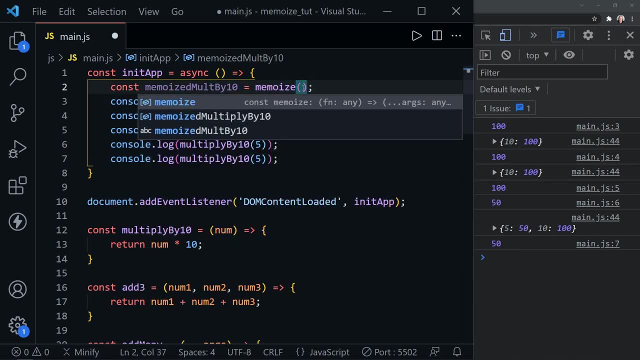 memoize, and we'll go ahead and pass in our multiply by 10 and now, with our memoized malt by 10, i'll select all of these and replace, and now we'll save and we should have the same result in the console that we had before. so let's go ahead and do that, and now we'll save and we should have. 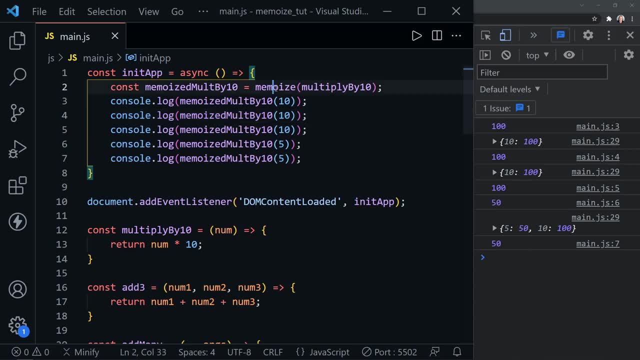 the same result in the console that we had before, but we're doing this a little differently now. we're using our memoized decorator function passing in our original function, which gives us a memoized version. so now let's go ahead and try this with add three. so i'll copy add three: 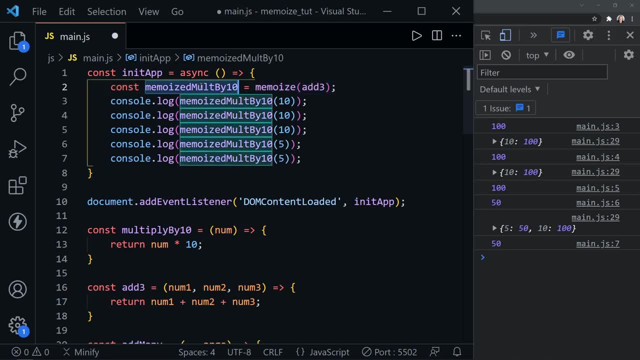 i'll pass it in here and i'll take this memoized malt by 10 and i'll just select all of them and we'll call this memoized add three. so we need three different parameters here. so i'll say one and two and i probably just should have selected all when i did that. but 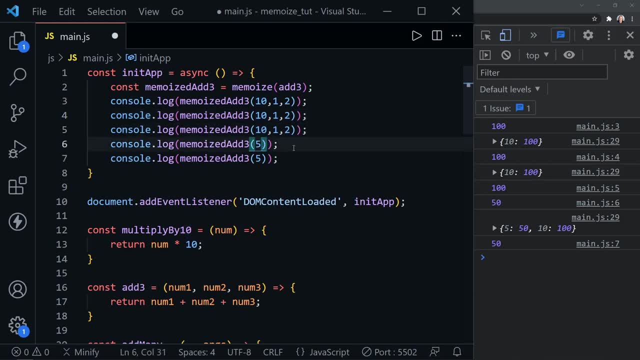 here we go, pass that in. now, here we'll go four and three, and once again four and three and save, and now we can see a different result because we're calling a different function. but it works with all the parameters. and here's what i really want to point out. is that the key? 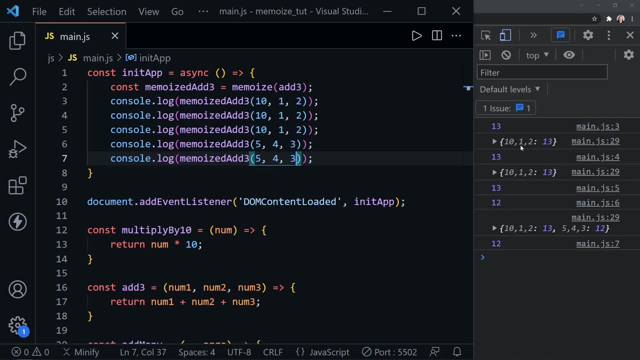 in our cache has all three numbers in it. it's 10 comma 1 comma 2, just like we passed in. so we're using all the parameters and then, when we go ahead and call the function with different parameters, notice it's got a second key in here, that's 5 comma 4 comma 3, and it's giving the result of: 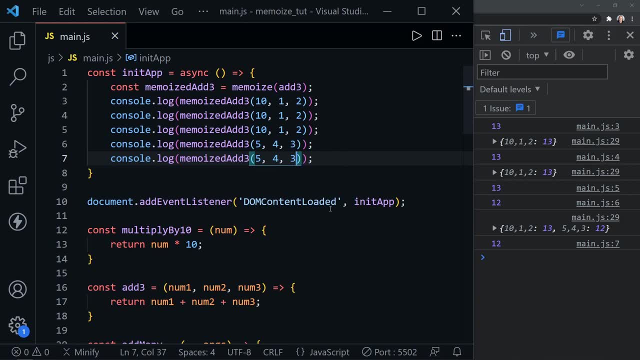 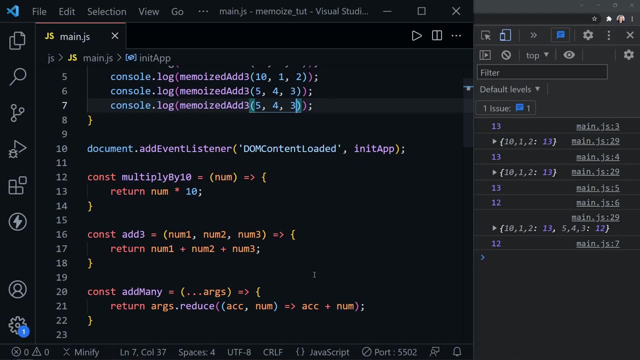 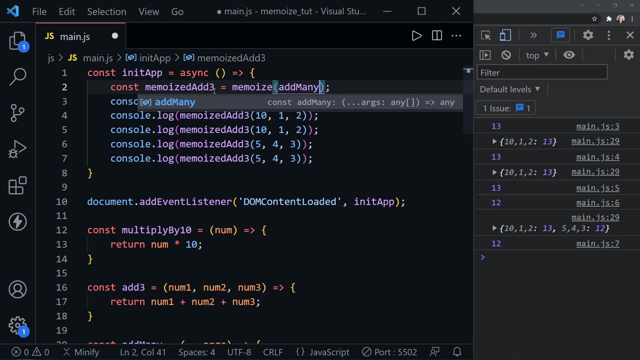 course of those parameters added together with add three. now let's go ahead and do this with add many and you can see it accepts args. then it uses reduce to add all of those arguments together. so now we'll take that and switch it to add many and here go ahead and select. 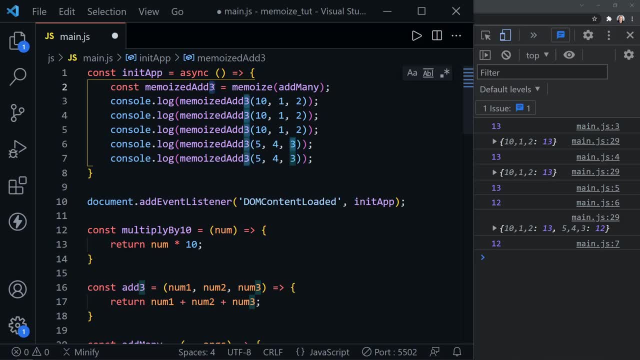 the three, because that's all we need to replace. oh, i had a three and one of the parameters, so we'll need to change that. but let's go ahead and select the three that have this, and we'll say one, two, three, four, five, and now i can't select these at the same time, but we'll say six, seven. 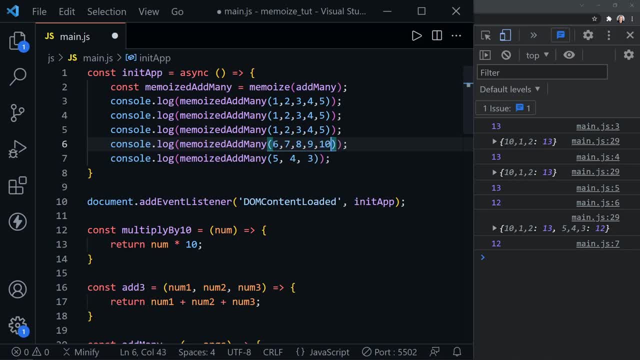 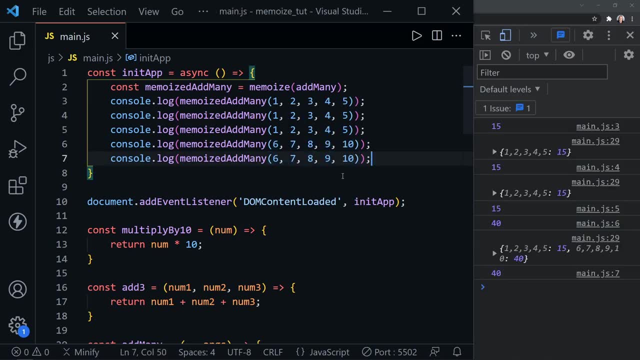 eight, nine, eight, eight a comma, there ten, and i'll just paste it in again here and now. we'll go ahead and save and we'll see the results of our add many. so the first time that memoized add many is called with one, two, three, four, five, it calculates 15.. the next time, 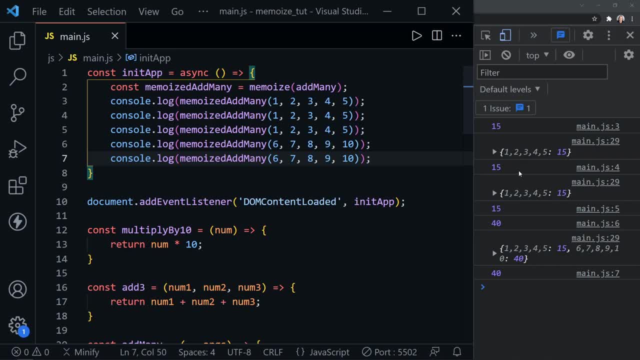 it gets it from the cache. and there's our key one, two, three, four, five and the next time it gets it from the cache again. now, when we call memoized, add many with six, seven, eight, nine, it calculates it and gets 40 the next time it looks to the cache. and you can see our second. 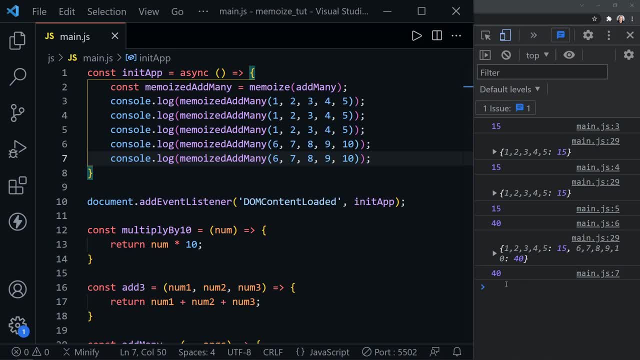 key in here with six, seven, eight, nine, ten, and there's the result, 40, and it instantly has it. now, before we finish, i'd like to go ahead and apply this to one processing intensive function, and there's no better way to do that than with recursion, and at least give example of it, and 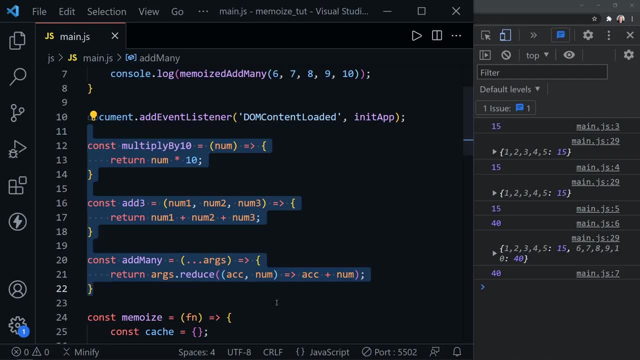 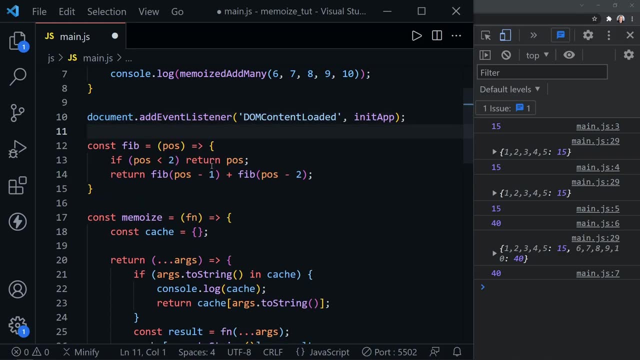 we'll get the classic example here of fibonacci. so i'm going to replace all these functions we have here and paste in a typical fibonacci function that's going to give us the fibonacci number that's in the sequence at whatever position we pass in. so i'll pass. pass in a higher number. 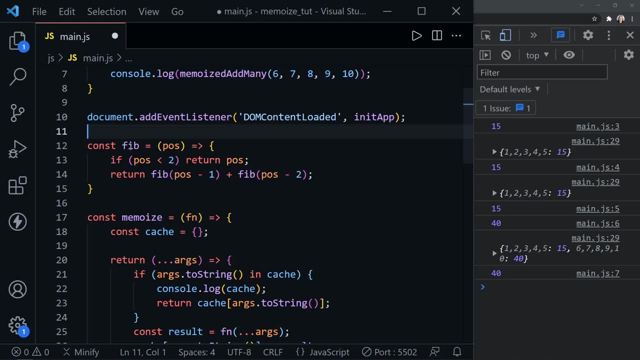 and, of course, take longer to calculate, because with recursion, which i also have a tutorial on and i will link to below- it calls itself. so fib is calling fib here and fib here in the function. so you get. so you get some intensive processing there compared to just your typical function. so what we want to do is: 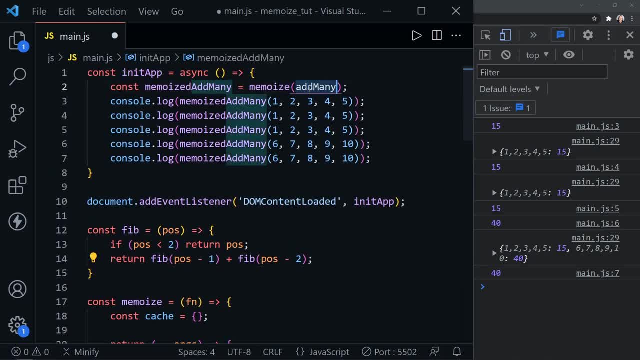 memoize that. so let's change this now to memoize fib and then we'll go ahead and select, add many here and i'll come down and just change that to memoized fib. now we just want to pass in one number and i think if we pass in the number 40, it's definitely going to take our process. 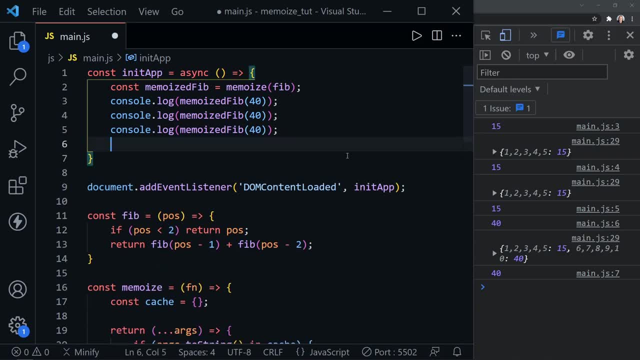 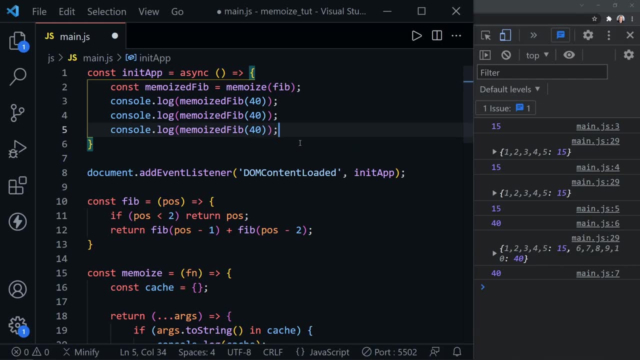 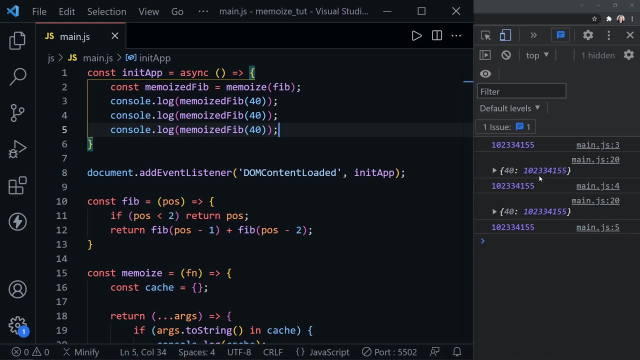 in, at least on my computer. it will take it a little bit to get that number. so let's see what happens now if we save and how long it takes to get each number. well, it took just a little bit, but after we got the first one right away, it was there in the cache each time. so if we went ahead, 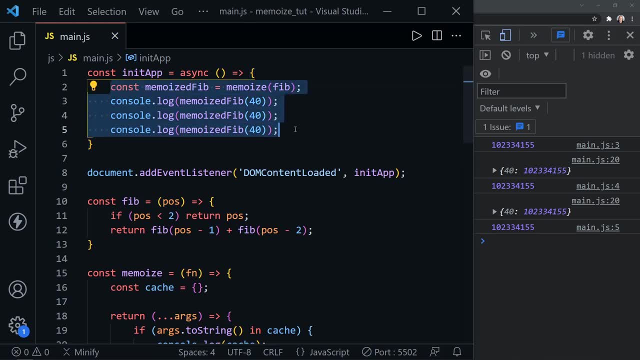 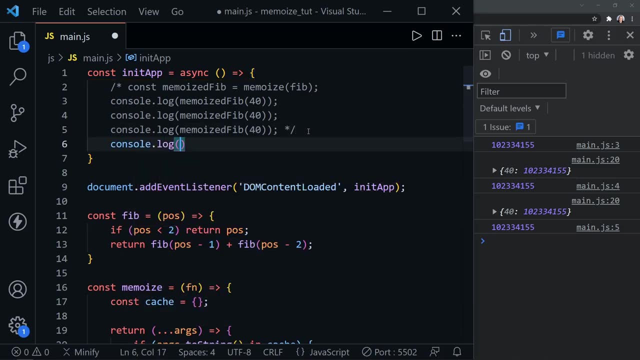 and compared this. let's go ahead and comment this out. and now let's just call fib three times and look at the data and see if we can get that number right. so let's go ahead and comment this out. and difference. so i'll say: consolelog, fib, pass in 40 and i'll put that in there three times. let's see. 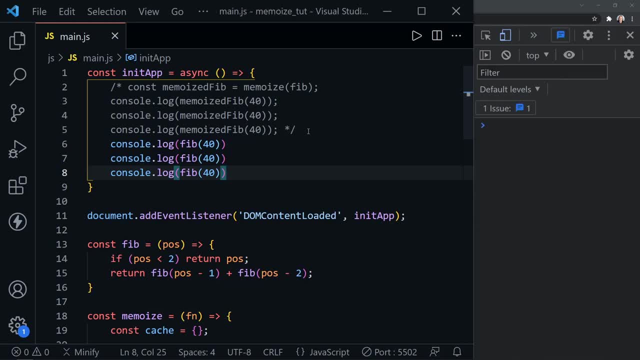 how long it takes now and we're waiting on the first one. now we've got the first one. now we're waiting again, there's the second and now we finally got the third. now, in comparison, let me comment these out and let's go back to how we originally did this and save. 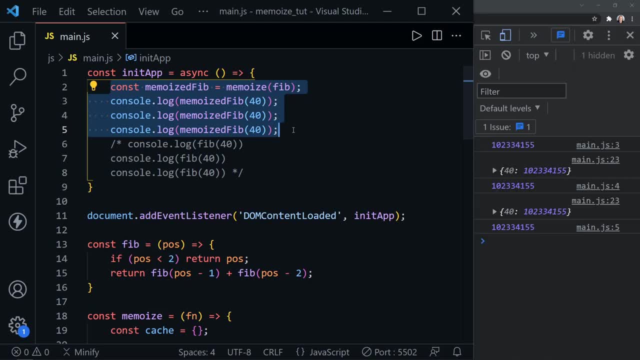 waiting on the first one and now we've got all three, because the other two are delivered instantly from the cache. and that is really the bonus of using memoize and memoization in general. it's the beauty of the whole concept is because you are trading a little bit of memory.